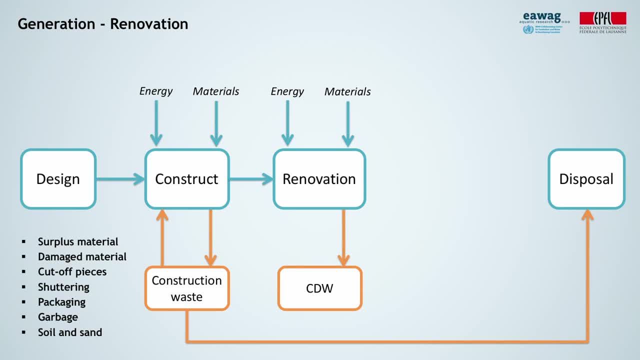 and demolition waste, which is comprised of all the previous materials, as well as rubble, gravel and mechanical equipment. Once more, part of this waste can be recovered or disposed of. Finally, demolition can result due to both natural disasters and man-made causes, such 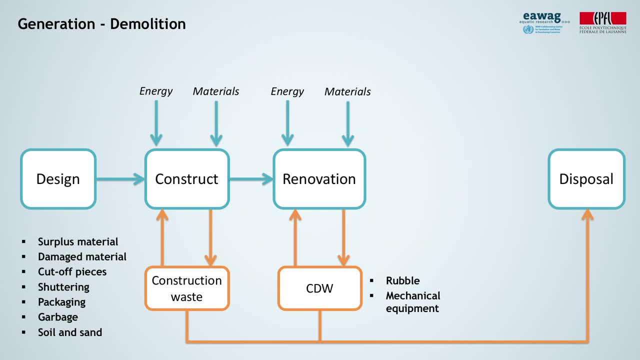 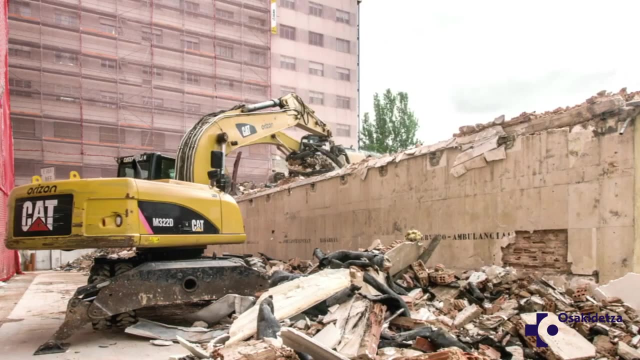 as civil conflicts and vandalism. Demolition produces a significantly different waste than construction or renovation. Demolition waste is composed of mixed rubble and debris, including wood, concrete, masonry and reinforcing materials such as steel, which can be contaminated by undesirable components. 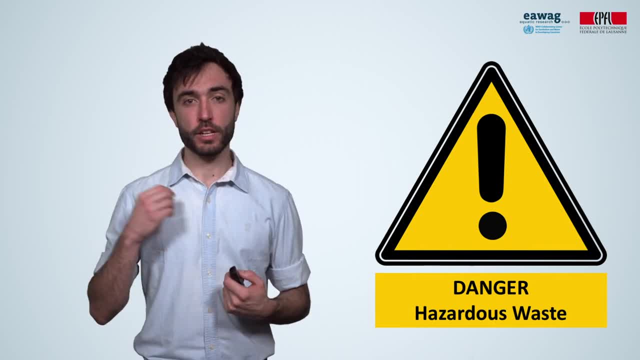 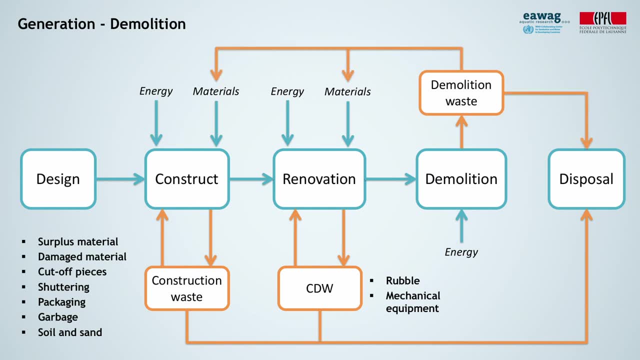 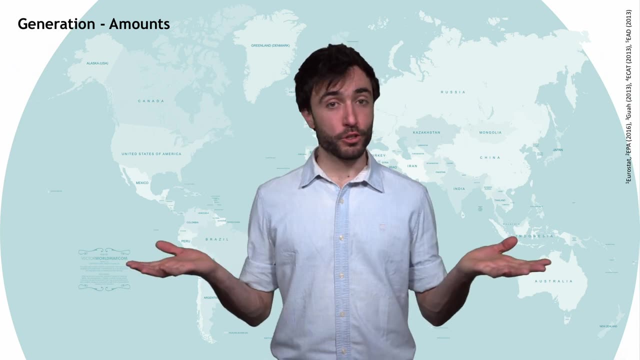 and or potentially hazardous substances such as lead, paints, stains and adhesives. This waste has traditionally been disposed of. However, it can also be reused to substitute virgin materials. So how much construction and demolition waste do we generate? Let's have a look to the generation rate. 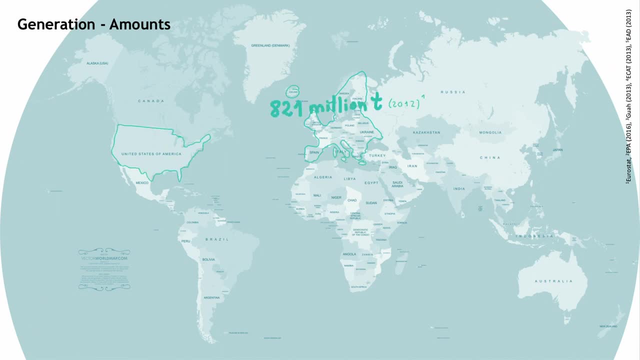 The generation rates of the European Union, United States, Japan, China, India and the Arab cities of Dubai and Abu Dhabi. The European Union seems to generate most construction and demolition waste, followed by the USA. Hmm, but what if we now calculate the per capita generation rates? 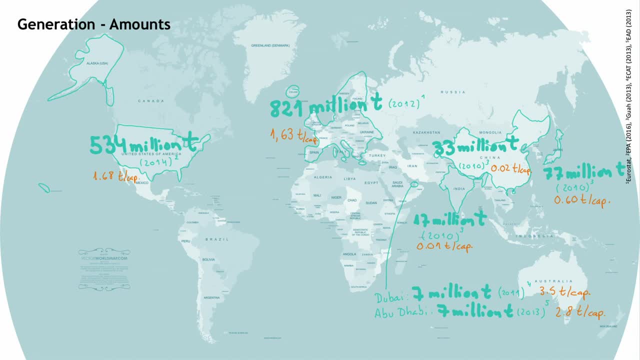 The per capita generation rate of the European Union is the same as the per capita generation rate of the United States. Wow, These numbers convey quite a different message. Note specially the high construction and demolition waste generation rates per capita of Dubai and Abu Dhabi and the low generation rates of China and India. 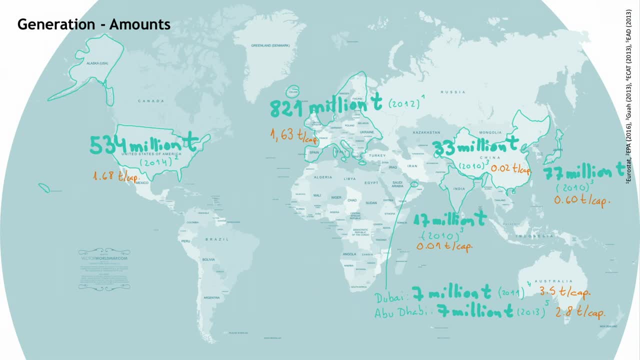 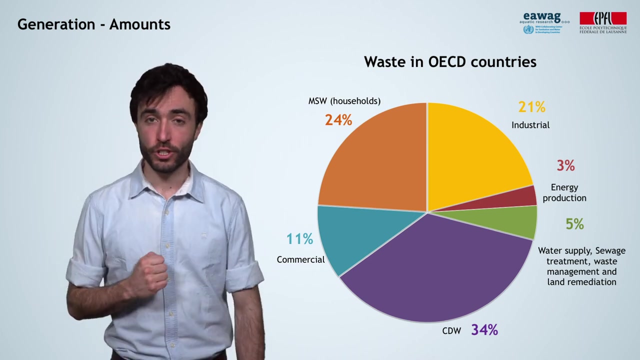 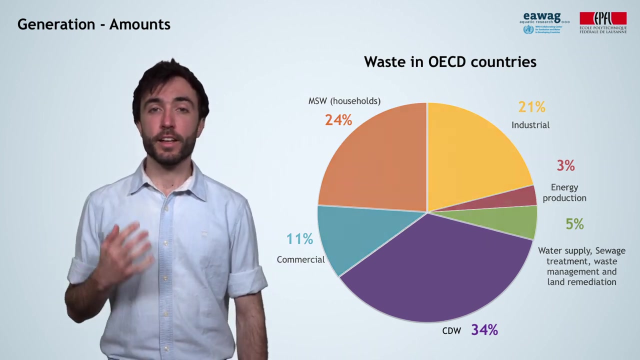 However, most published figures are mere estimates and often countries do not report their actual generated amounts. Therefore, these figures need to be interpreted with caution. What we do know is that construction and demolition waste often represents the largest proportion of total waste generated in weight. 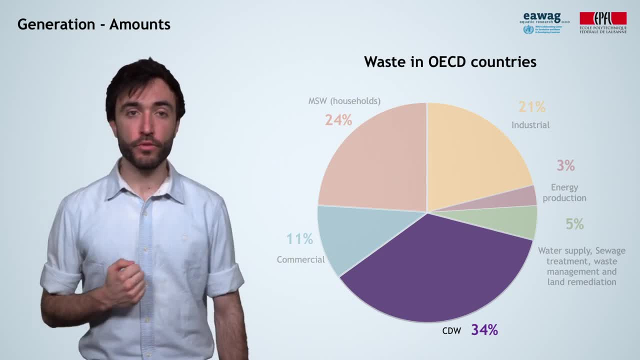 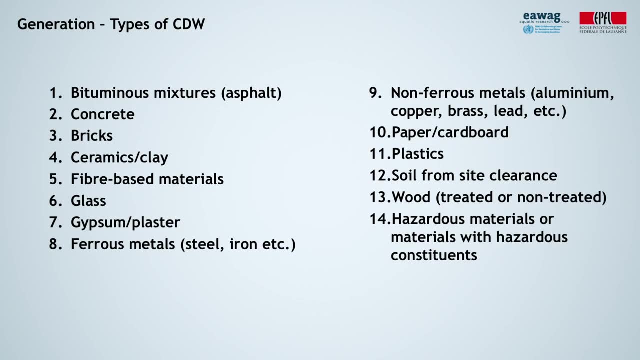 In OECD countries, for example, it accounts for 34% of the urban waste generated. as shown here, In terms of the individual components, we consider these 14 categories of materials as the main constituents of construction and demolition waste. Thank you for your attention. 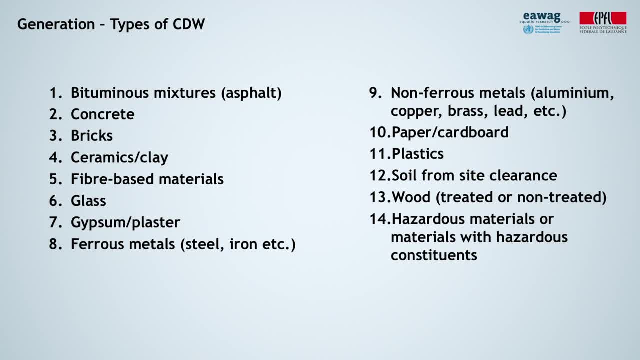 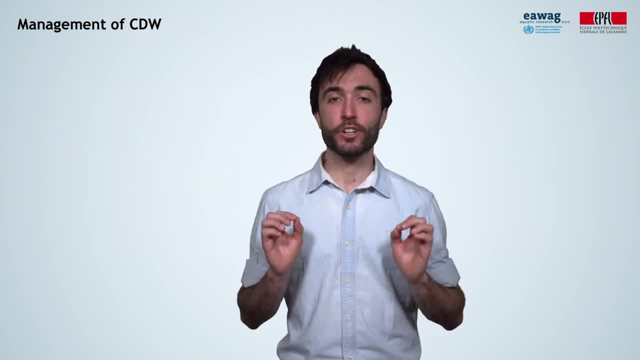 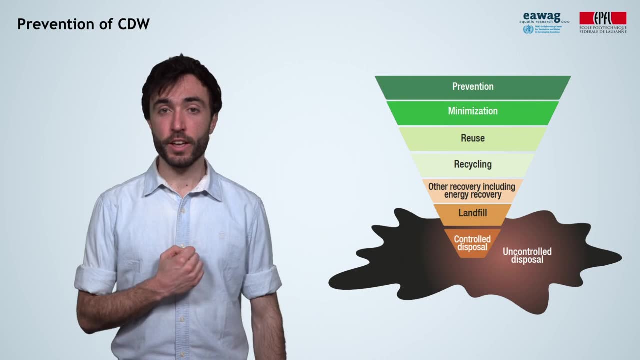 You are welcome to stop this video for a second to have a more detailed look at the list. Let's have a look at some important concepts when managing construction and demolition waste. The very first step, as indicated in the waste hierarchy, implies preventing the waste. 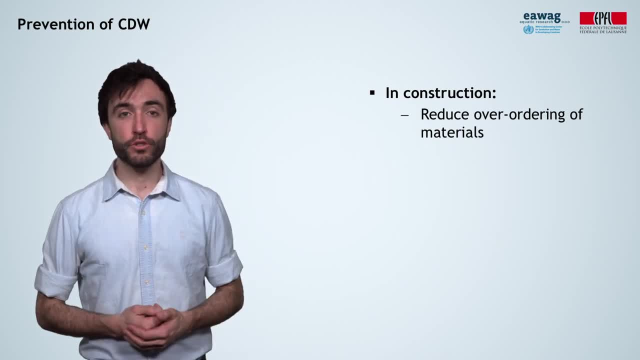 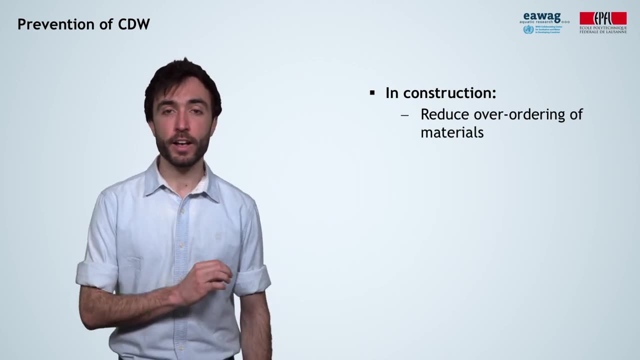 A simple measure to prevent waste during construction is to reduce the over-ordering of construction materials. Prevention during demolition has a very important role In the case of construction and demolition waste. construction and demolition waste is a very important component of the design of the buildings and therefore requires thorough. 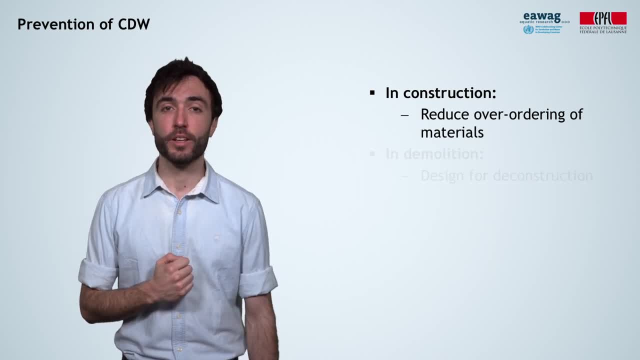 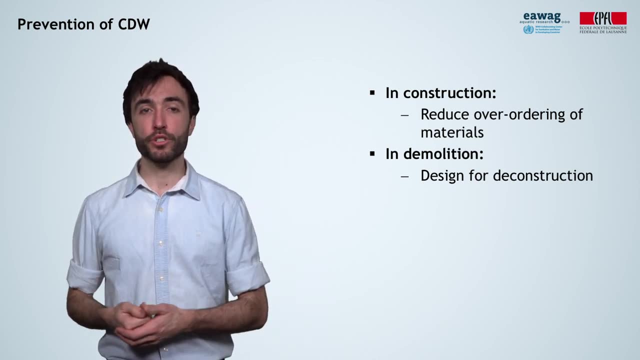 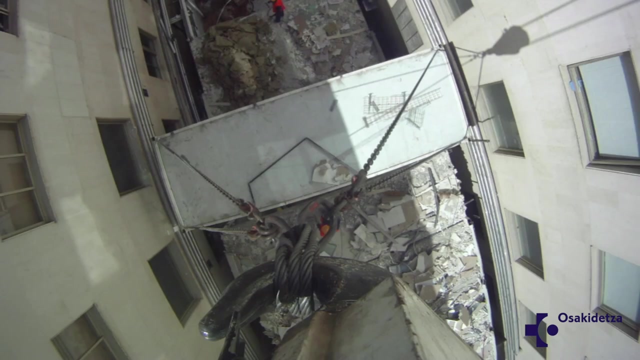 and timely planning already in the design phase. When buildings are designed for deconstruction at the end of their life cycle, more components can be reused and it prevents a lot of demolition waste. For instance, here we see the deconstruction of a modular building where the different 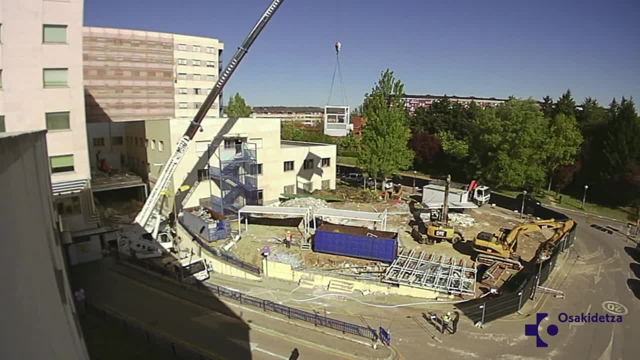 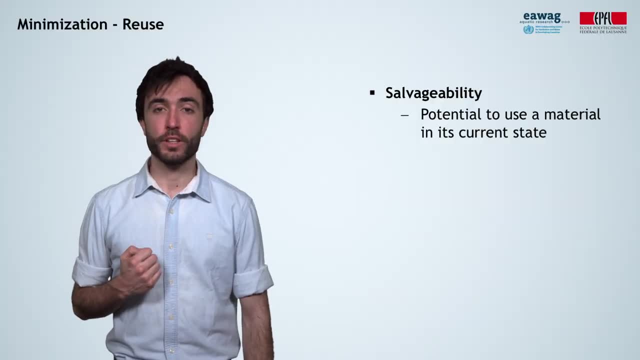 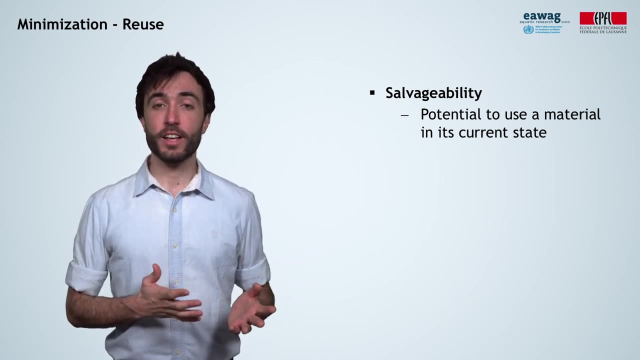 modules can be dismantled and their parts stored for further use. The construction of a modular building is a very important part of the design of the building. When talking about reuse of construction and demolition waste, we use the term salvageability. The salvageability of a material is defined as its potential to be reused in its current. 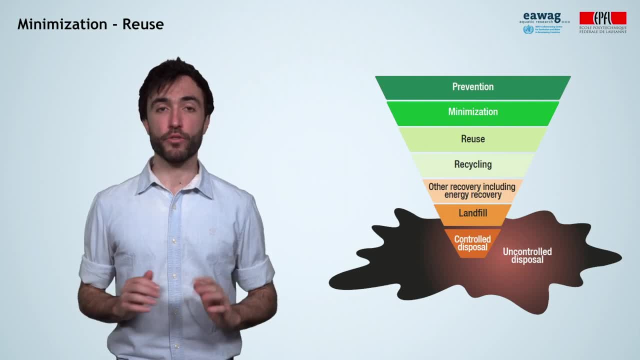 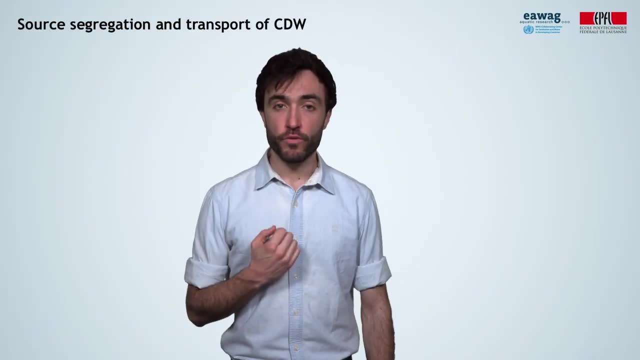 state, minimizing the needs for transport and further processing. Some debris might be used for backfilling of holes, for instance. Due to the variety of waste materials, There's no way of removing them. This is very important to segregate construction and demolition waste. 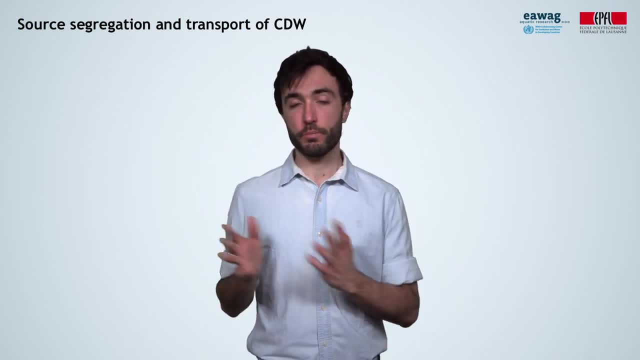 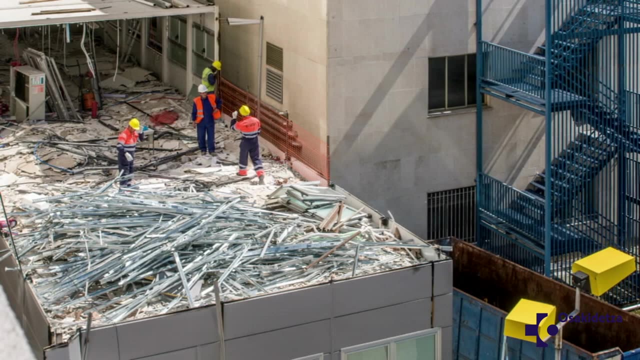 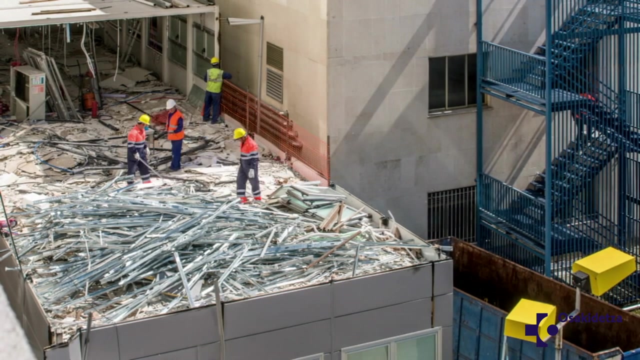 This can be done at source, ideally, or in specialised treatment plants. This way, each waste stream will be managed as required. Here we see how these operators have separated out all the metallic frames of this soon-to-be demolished building. Then the materials need to be transported to the demolition site. 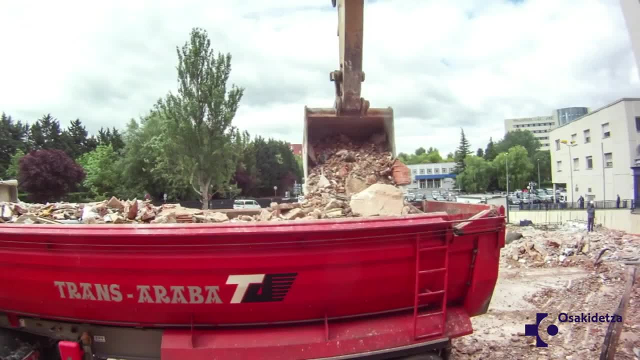 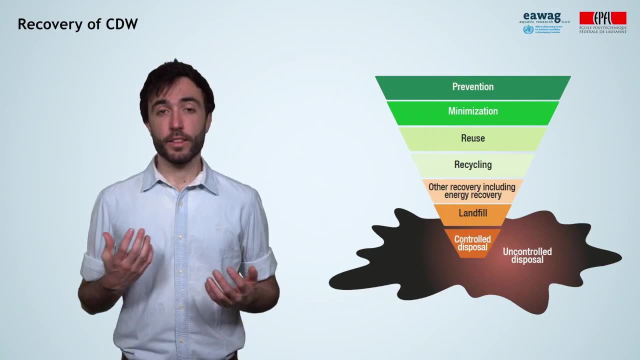 The bulk of the materials, the new materials, are stored here, And that's what we want to make, So each one has a separate storage area, ideally a processing plant for further reuse or a final disposal site. The next step in the hierarchy is to recycle or recover any materials. It is important to mention.